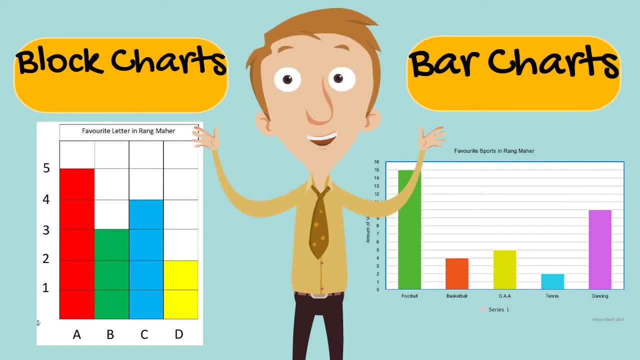 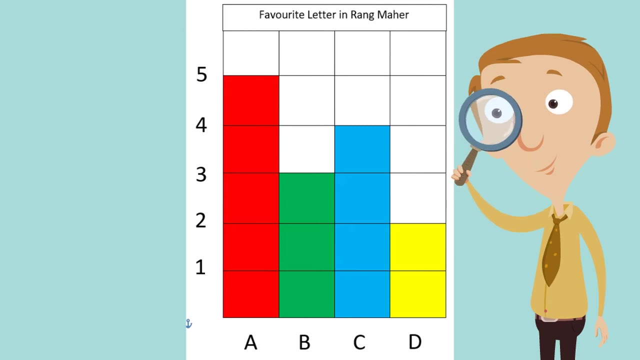 One of them is called a block chart And the other one is called a bar chart. Let's take a quick look at block charts first. These are quite like pictograms, but instead of pictures showing the data, there are blocks like these. 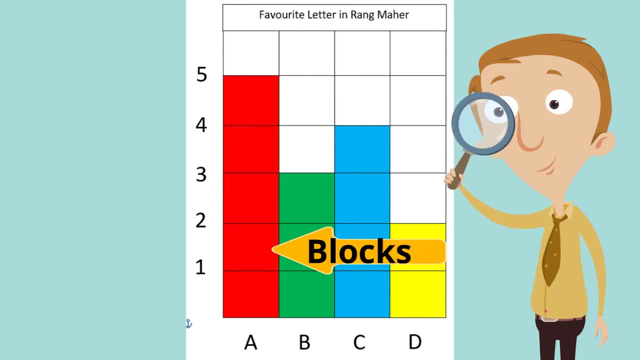 Block diagrams are good. if you have a small set of data to show on a chart, It gets pretty hard to count all the blocks if our numbers start to get really big. Block charts have a title Up the top. that tells us what the survey question was. 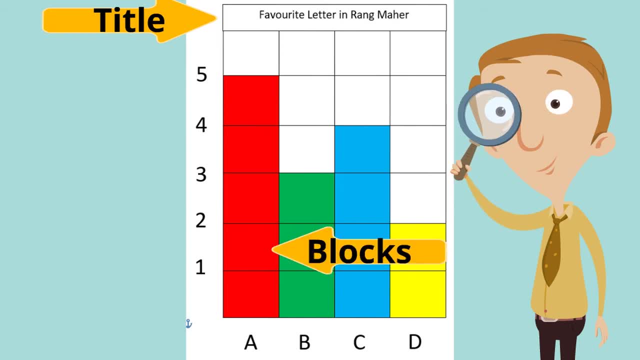 They've got the blocks to show how many votes for each. They have the labels down the bottom to show us what people answered in the survey. Block graphs are pretty basic and we usually use them when we're first learning about data in second class and in third class. 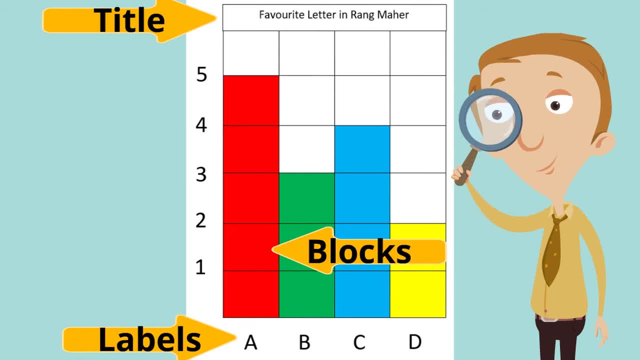 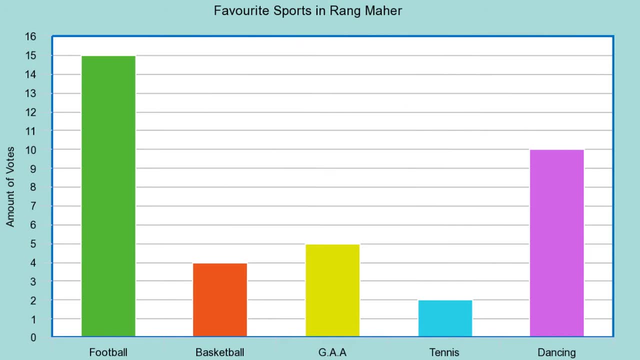 So we're not going to spend too long looking at them. Instead, we're going to jump straight into the survey. We're going to start with the first class. We're going to start with the second type of chart, a bar chart. 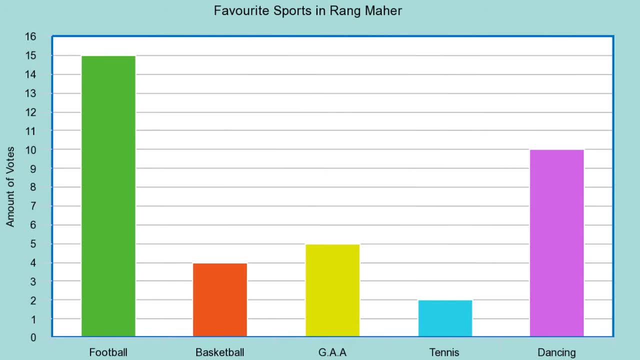 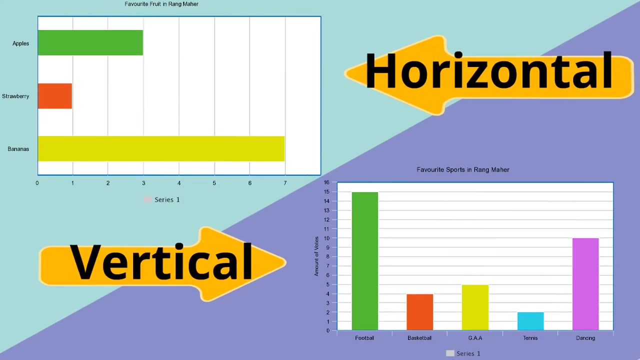 Bar charts are different. Instead of counting blocks or pictures, we read off the scale on the side. Bar charts are much better at showing big groups of data because you can quickly see how many are in each group by reading across to the scale. Bar charts can be drawn horizontally. 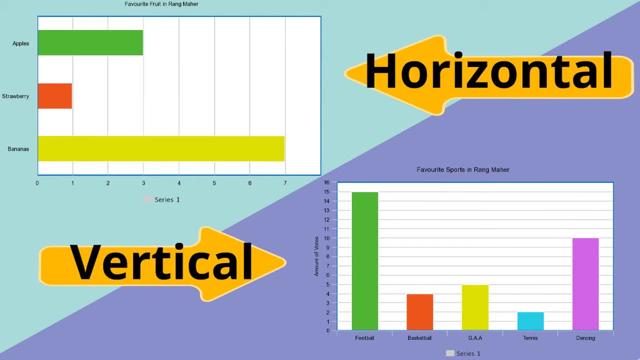 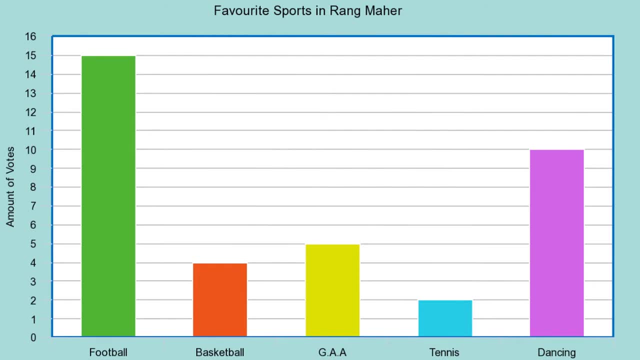 That's from left to right, like in the top one, Or they can be drawn vertically from top to bottom. When we're drawing bar charts, being careful and accurate is very important. There are certain parts of a bar chart that have to be there. 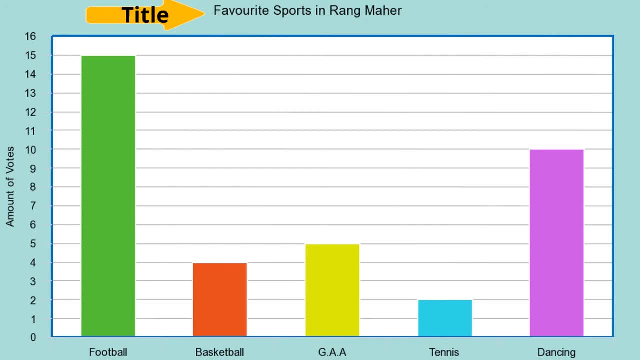 The title up the top tells us what the survey was about. Its scale on the side On the side tells us what we're counting up in. It's also how we read how many votes each group got. The bars show us how popular or unpopular each group was. 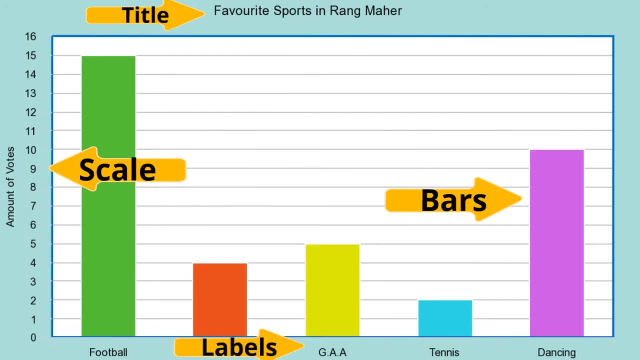 And the labels down the bottom tell us what options the people were given. Watch what happens if we take away any one of these four parts, If we take away the labels. well, we know that this is a survey about favorite sports, but we have no idea what the green bar, the red bar, the yellow bar, the blue bar or the purple bar stand for. 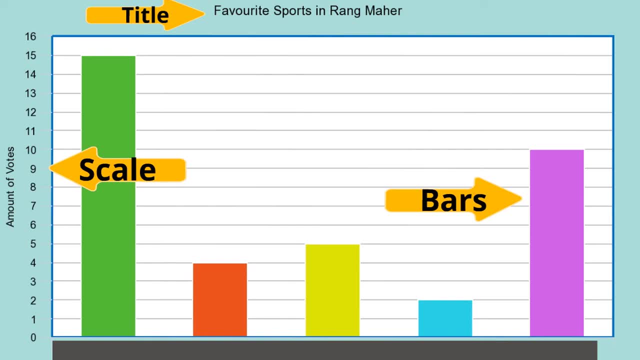 We've no idea which sport is which, So we can't really answer any questions. If we took away the scale on the left hand side, well, we have no idea how many people voted for each. We know it's a survey about the favorite sports. 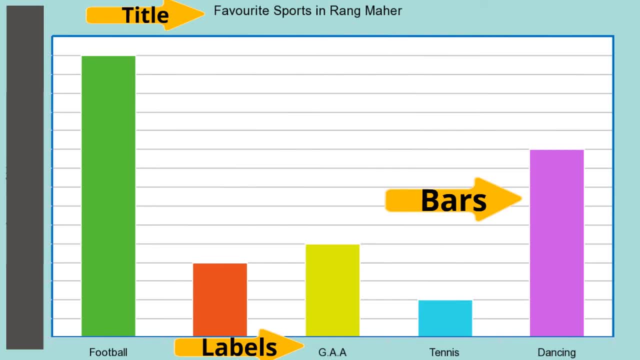 We know the sports that were chosen, but we've no idea how many people voted for each. So, again, not a very useful graph. And finally, if we took away the title, well, we know this is a survey where the answers were football, GAA, tennis, basketball, dancing, but we've no idea what the question was. 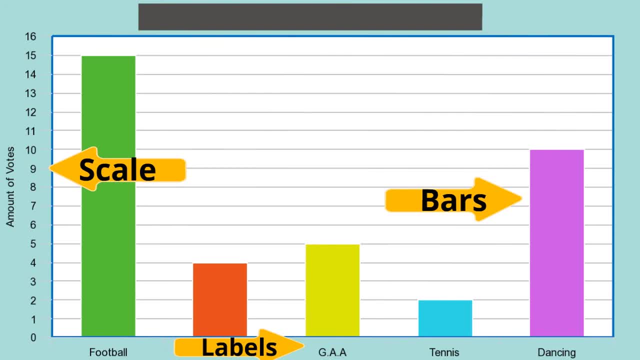 So again, not a very useful graph. That's why all four parts are different Parts. title, scale, bars and labels are all equally important. Have a look at this completed bar chart. Can you think of two questions you could ask about this bar chart? 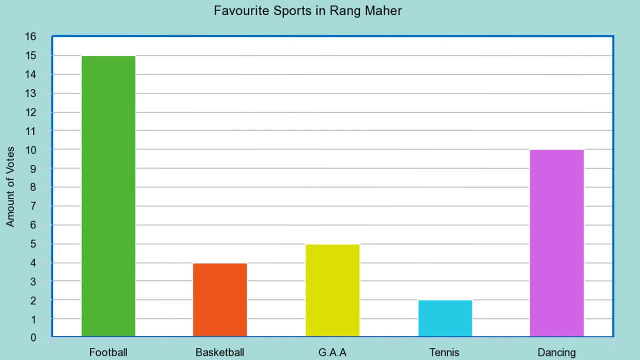 Pause the video and write down two questions. Well, you may have already put down some of these questions, but let's try answer these ones anyway. Question one: What is the favorite sport in Rongmar? Pause the video and write down your answer. 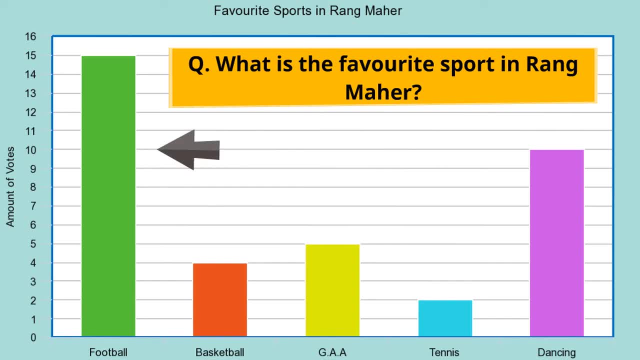 Well, the answer is football, with 15 votes. Question two: How many people voted for dancing? Pause the video and write down your answer. Well, the answer is 10.. And we figured that out by reading all the way across to the side.